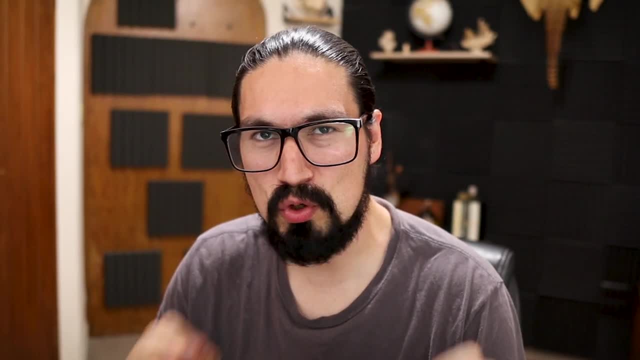 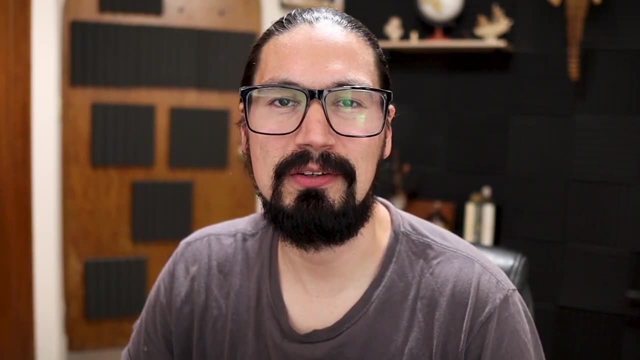 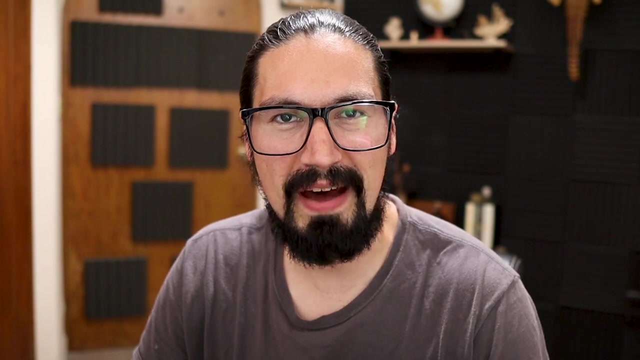 focusing our attention into which process or chemical engineers should or not learn Python, but mostly what we're going to be doing is to see the applications of Python in chemical engineering or overall in the chemical industry, And for this, what I would really love to do is to first define 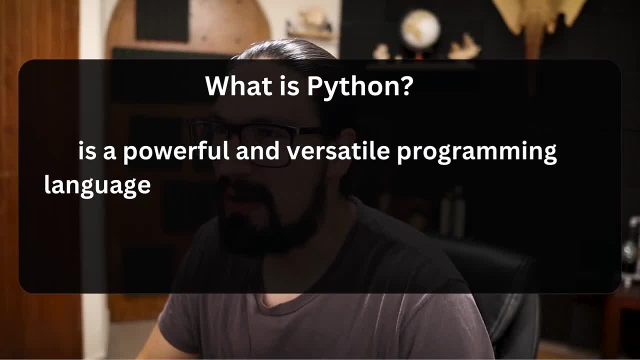 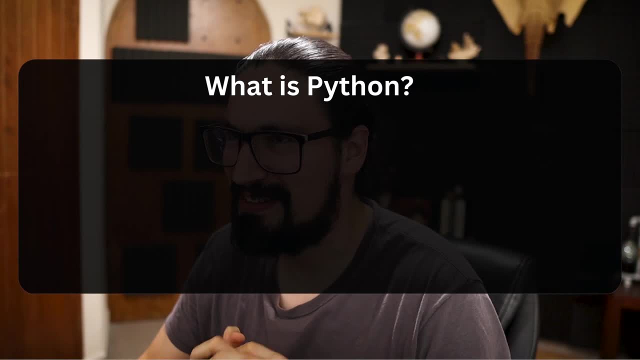 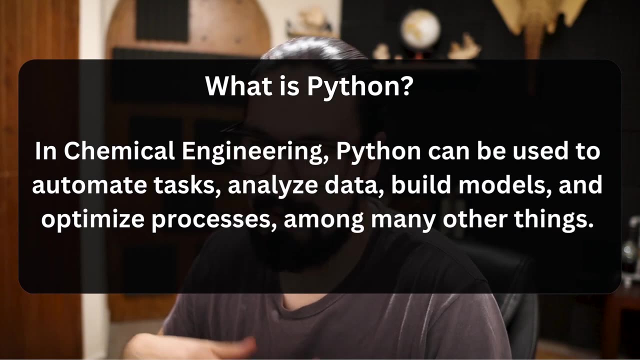 what is Python? Python is a powerful and versatile programming language that is widely used in many different fields, including science, engineering and data analysis. In chemical engineering, Python can be used to automate tasks, analyze data, build models and optimize processes, among other things, for sure. 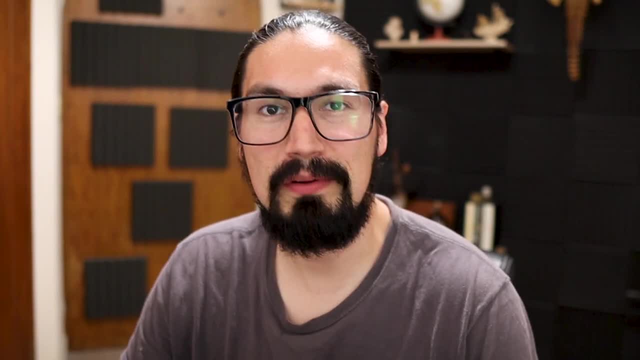 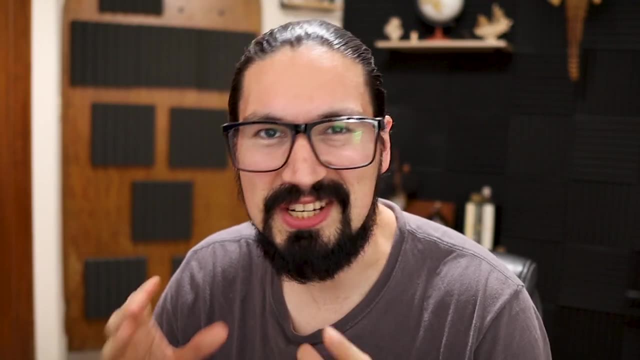 Remember that programming languages allow us to build software, build stuff, and the applications are limited as our creativity. But of course I'm not going to be mentioning all those niche applications. I'm going to be going straight forward into the main applications of Python. So if you already 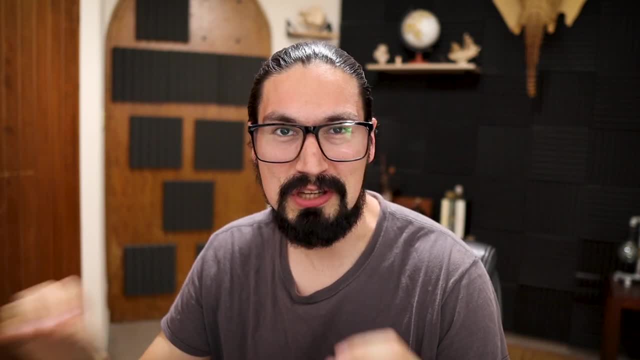 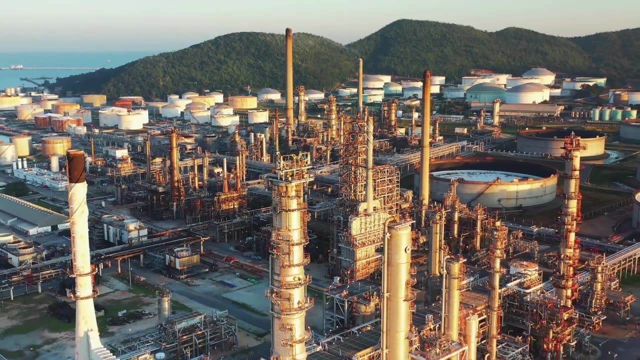 learned Python. great for you. You already know certain type of applications, But if you're wondering whether or not you should go for Python, or maybe you are not quite sure how this programming language applies to the chemical industry, this is the video for you. Let's get started with the list. 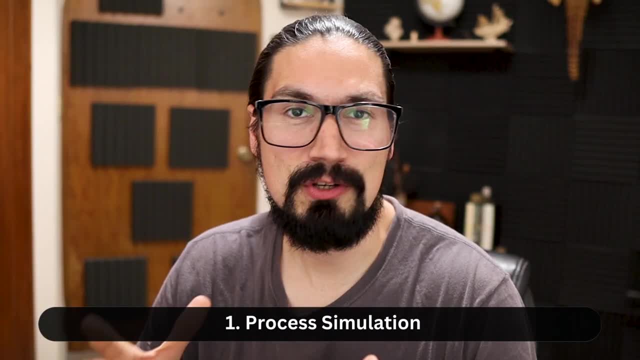 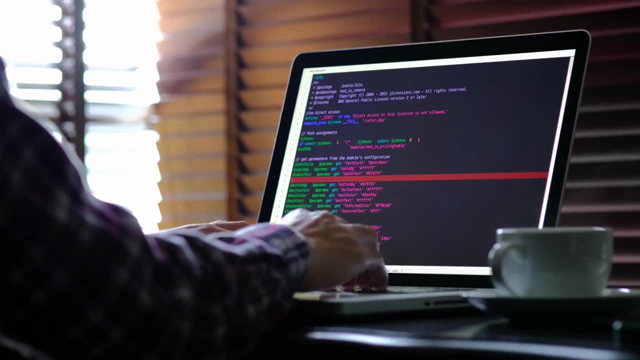 Number one will be process simulation. Yes, as you can imagine, guys, we can build a software that will calculate certain type of inputs and outputs, or maybe will allow us to literally simulate a unit operation. Maybe we're talking about a heat exchanger that you have on. 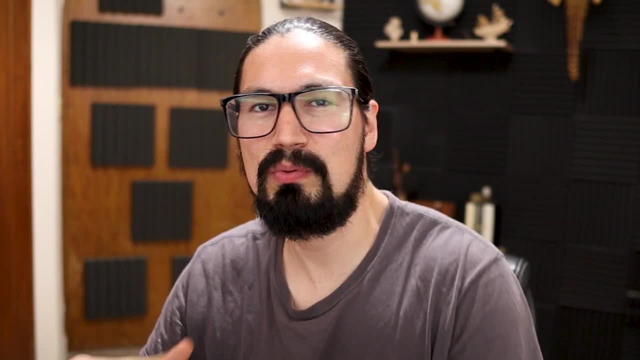 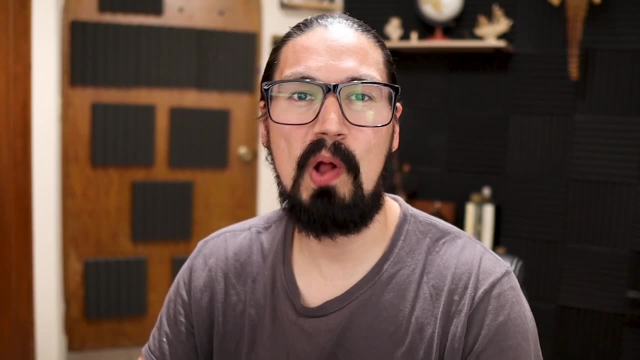 your own chemical plant and you don't want to be simulating this with other expensive tools. Maybe you want to apply your own software for your unique needs. One of the best things here is that you can always customize or add or remove certain type of features. that will help you to improve. 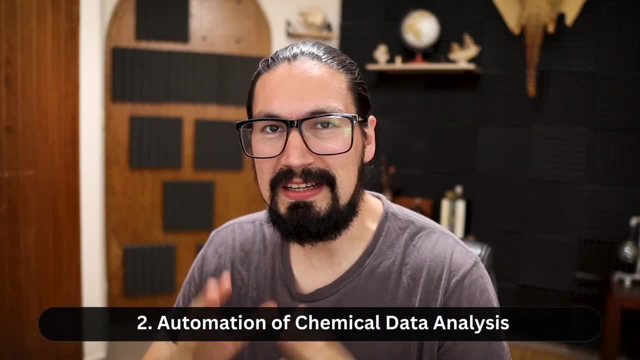 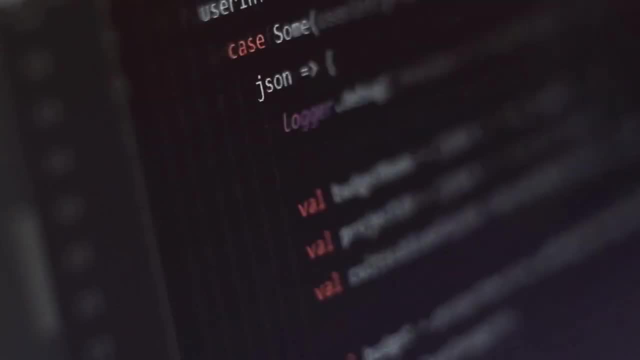 your process engineering work. One of the things that I really really love is automation. Making a computer work for a computer is a really really important part of the process engineering process. You don't need to be wasting time moving through the computer or software and knowing that there 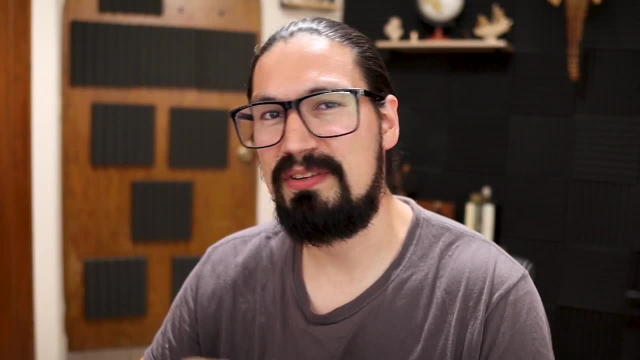 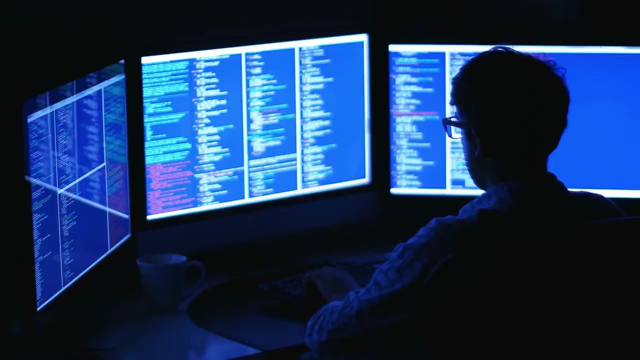 will be no human error. There are many ways in which you could be doing certain type of automations, but I'm going to be talking about automation of chemical data analysis, And what I'm talking about here is that maybe, as a human, it will be virtually impossible to keep track of. 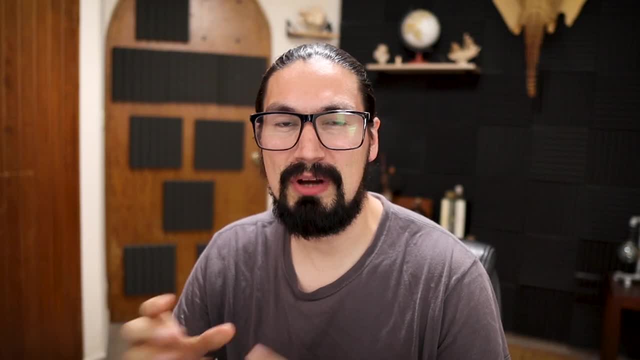 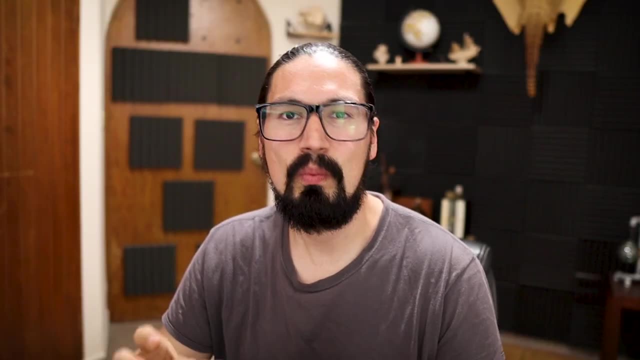 I don't know, maybe 100 variables and interrelate them, trying to make sense, understanding whether or not those are correlations or causations, and trying to improve. which type of conditions are going to be improving the process? which type of conditions? 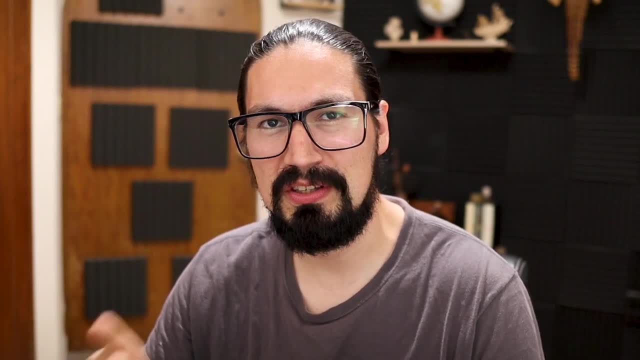 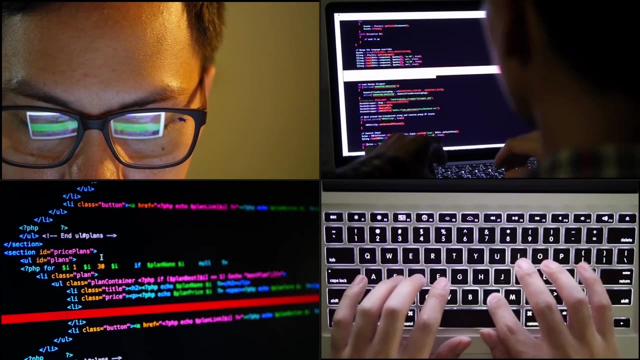 are not going to be helping us at all, or which type of changes into the input are actually irrelevant. But with Python we can keep track of all this data and be able to automate all this work, all this analysis and essentially being able to get a final result in this big chunk of 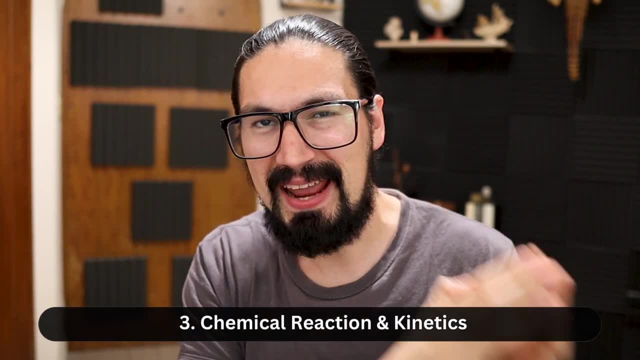 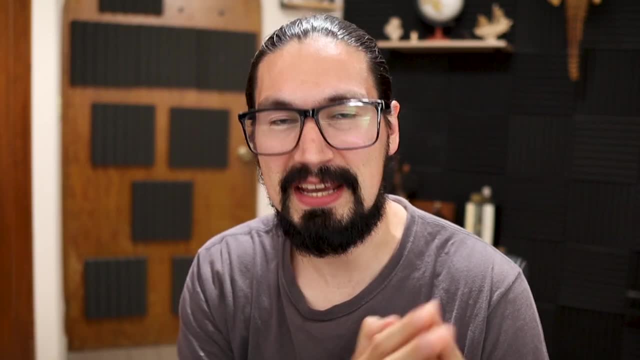 data. Python can be used, as stated before, in any type of unit operation, But I really want to remark that Python is really great at automating the process engineering work. It's really really great when you are doing calculations, for instance, in a chemical reactor in which you 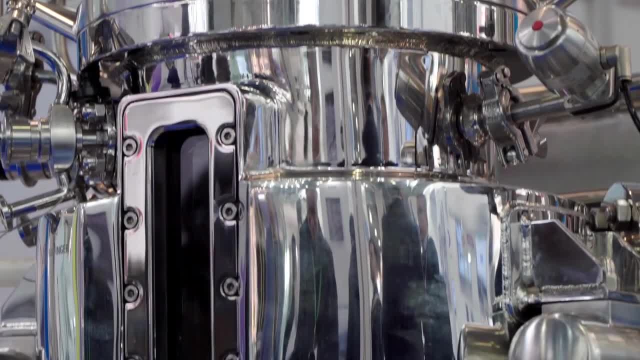 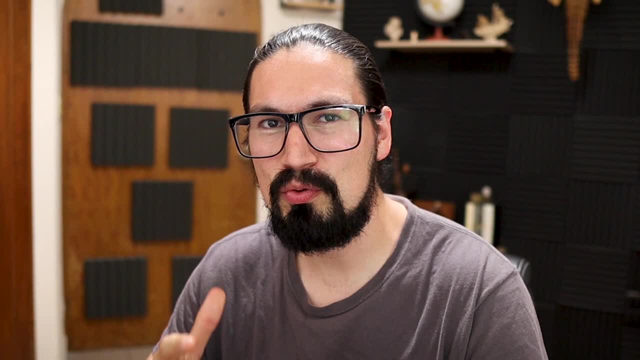 could be adding or removing certain type of conditions. Maybe temperature, pressure, concentration, flow, risk conversion will be, for sure, something relevant. But what I'm talking about here is trying to push the envelope, trying to model or simulate the kinetic model or the rate. 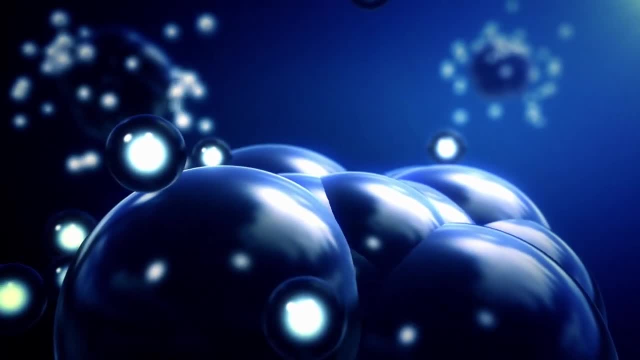 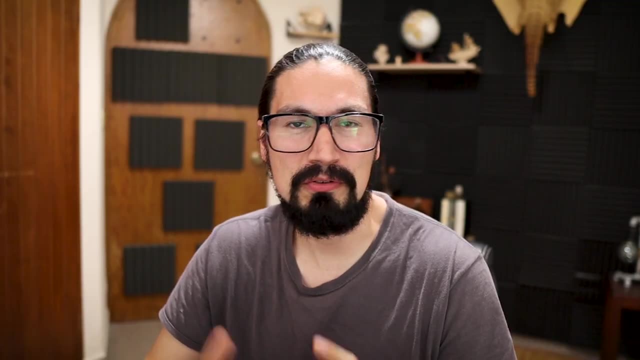 of reaction of certain type of components or chemicals will be something that you should consider. Not only that, guys. if you're specifically talking about chemical reactors, you will be able to size it. you will be able to understand how heat affects your reactor. 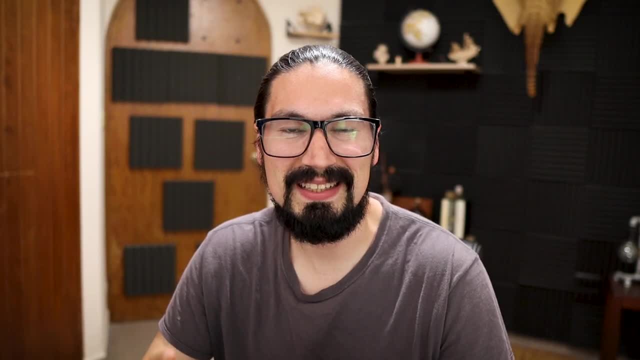 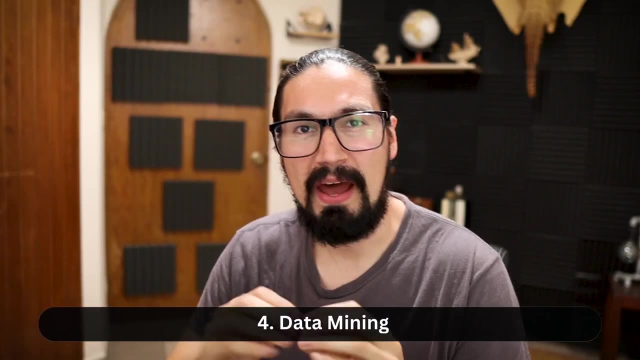 you will be able to model the flow rates and, more importantly, being able to predict the final results or the final product conditions. Another application of Python will be data mining, And, although it may be pretty similar to the one that I told you about automation, data mining is. 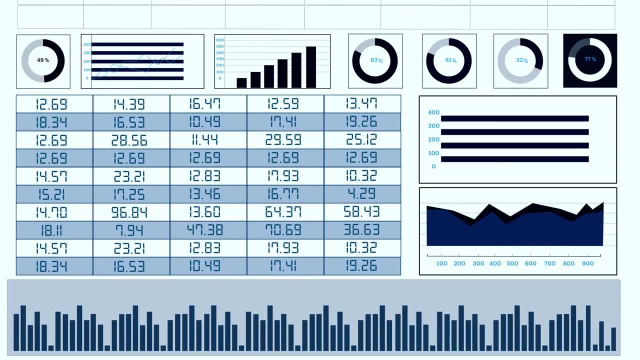 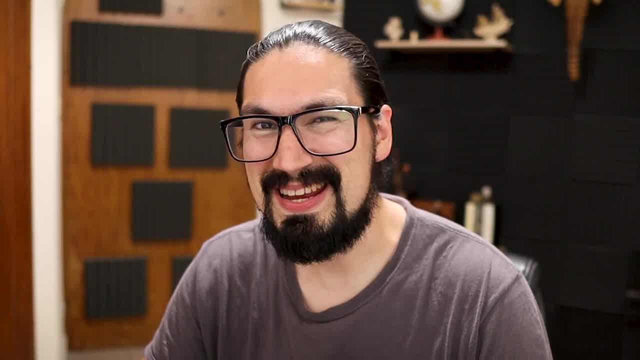 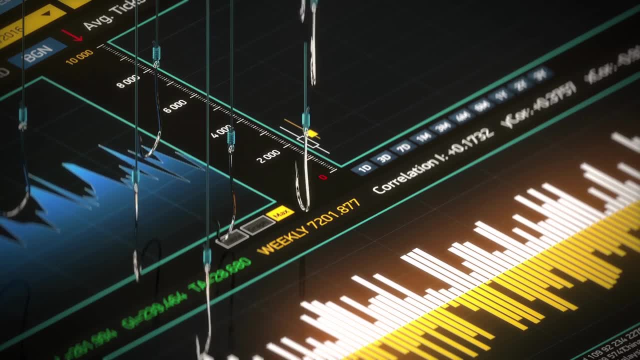 specifically done with the intent of looking for a certain output from a very big, very big, big, big database, And whenever I say big, I really mean big, like huge, like really literally databases of databases or a lot of data points that interconnect with each other that simply will not be able to be analyzed in a 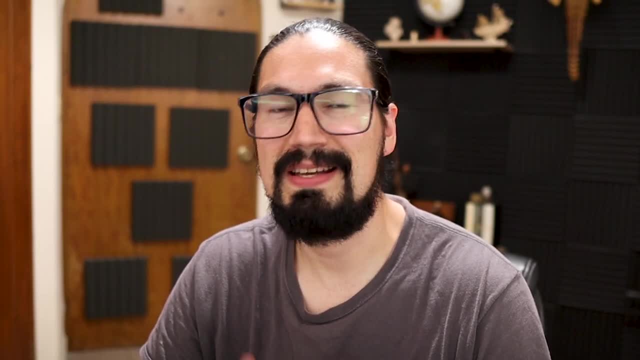 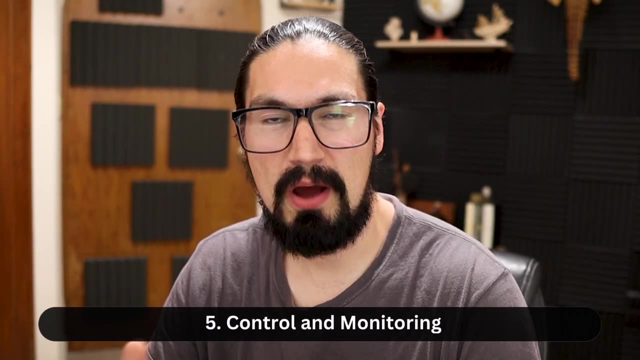 pivot table or in a spreadsheet. The main idea here is to, as the name implies, being able to mine relevant data from these databases. Control and monitoring of the process itself, or the conditions, is, for sure, something that you can do as well in Python. But more importantly, 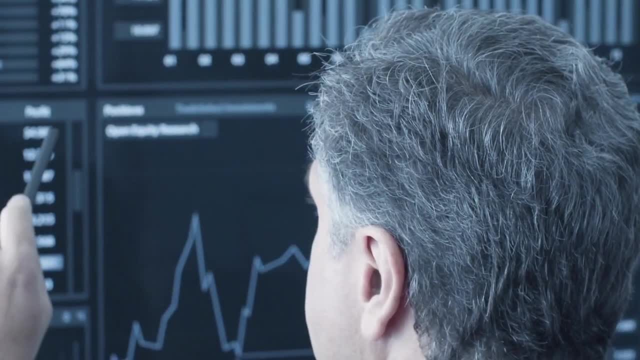 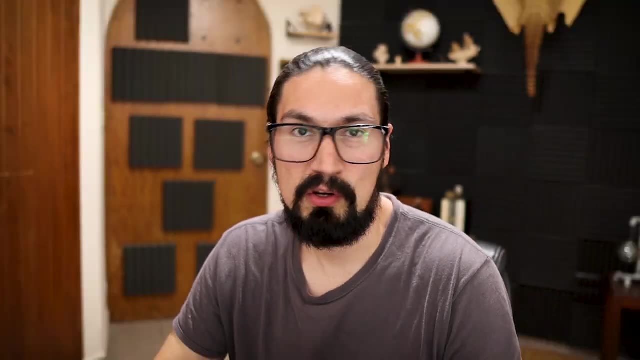 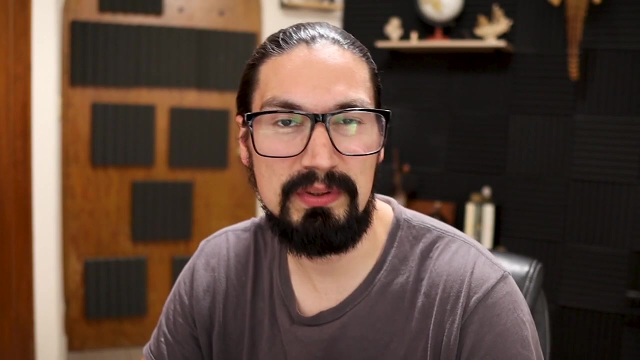 it's something that will allow you to improve the process conditions. With this software, you will be able to adapt control loops or maybe even improve certain type of control loops. Not only that: if you're talking about automation, maybe you want to improve the response of certain type of input variable. you want to verify whether 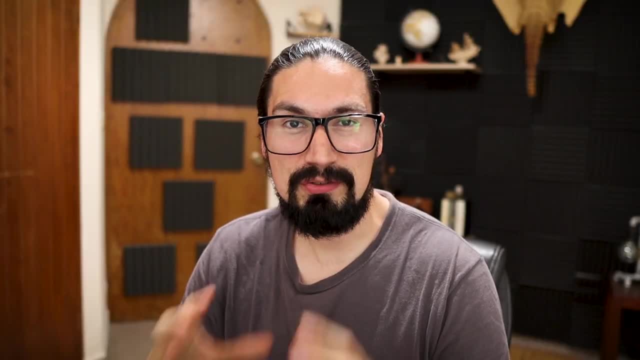 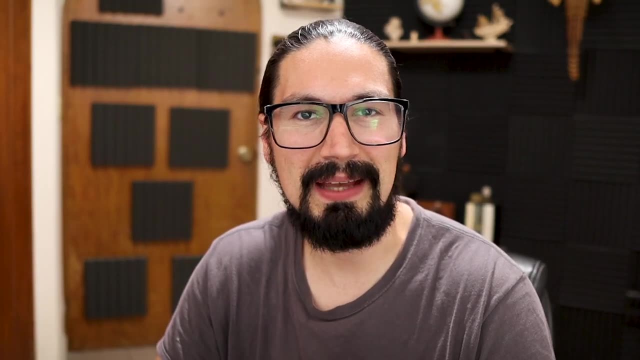 or not. the output variable will stabilize in certain time, And Python is really great at doing this. So whenever you go and take out your control or automation class, ensure to check out the applications of Python into the current software that you're using already. 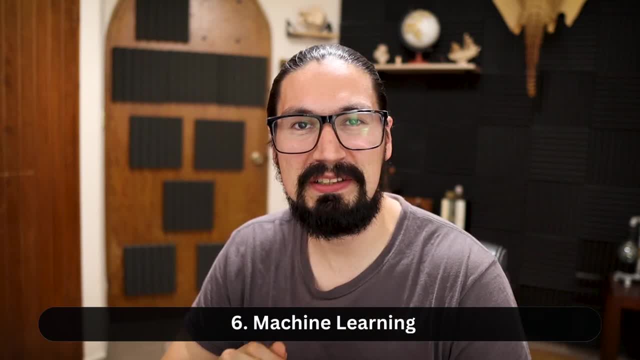 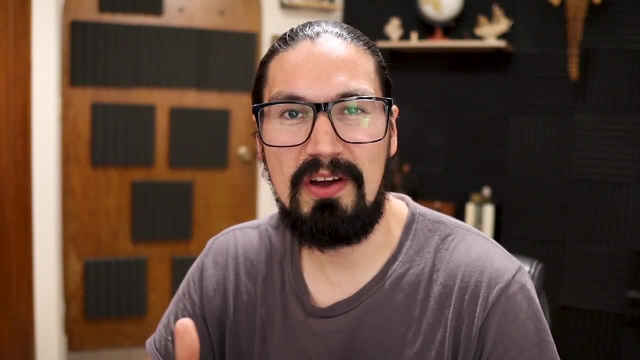 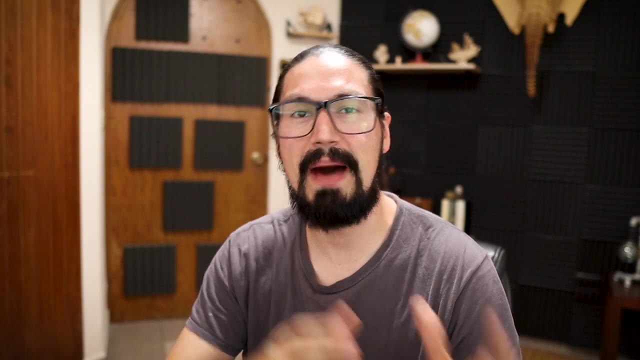 And finally, guys, machine learning. I actually have a machine learning video, so go and check it out if you want to learn the applications of machine learning in the chemical industry. But we never actually thought on how we do those type of machine learning softwares or algorithms, And what we're going to be doing here is, yes, using Python as a 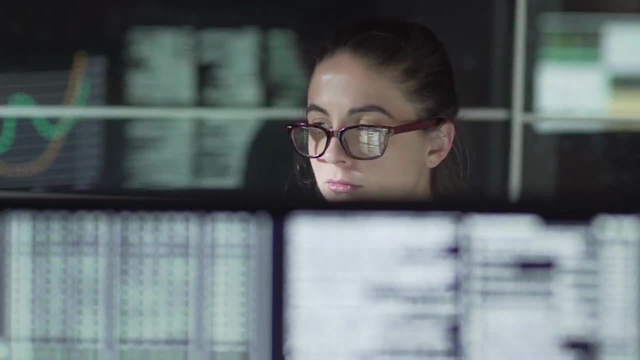 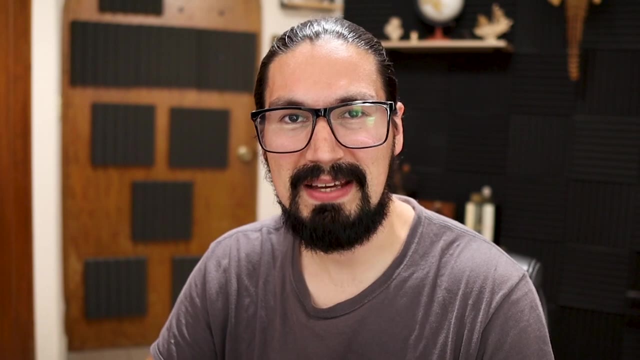 programming language to give instructions, to create a software or an algorithm that will be learning from the input data. Essentially, what we're going to be doing is to make our machine to learn For sure. you need to have a lot of logic and understand all the current models. 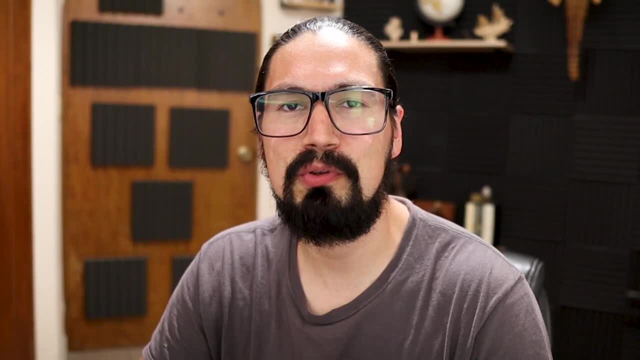 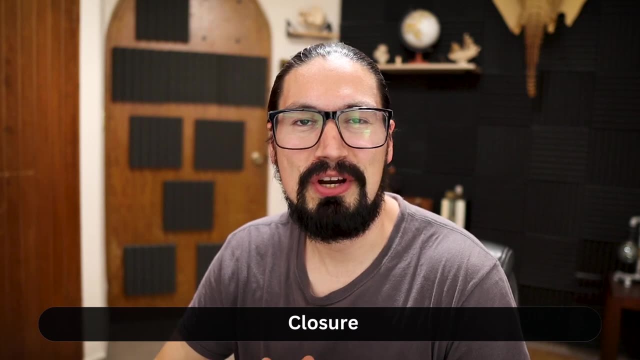 of machine learning, But with the help of this software, you will be able to get started with your machine learning software. And yes, those are certain type of applications I wanted to share with you guys. For sure, there are a lot of applications, As I said before, literally. 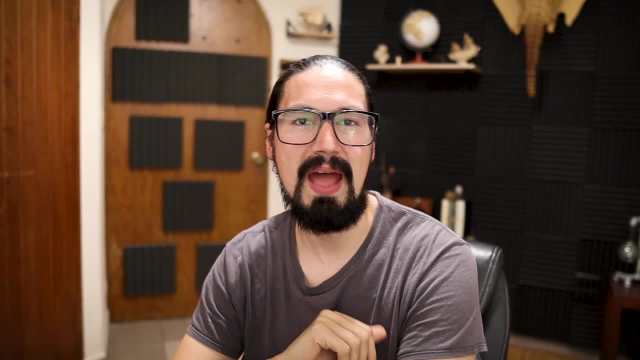 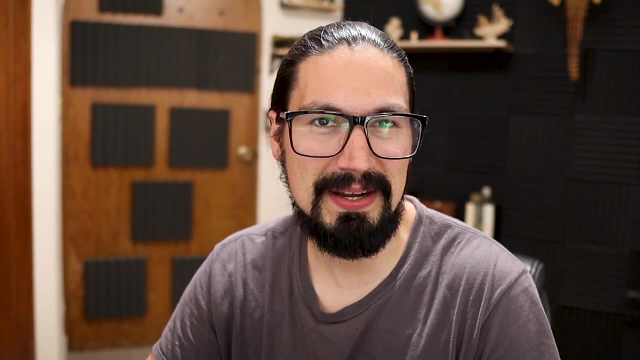 your creativity is going to limit all the applications that you may have as a chemical engineer. And for sure we already know that programming is powerful, but Python makes it easier for the chemical engineer. So, yes, I will say that most of the time. 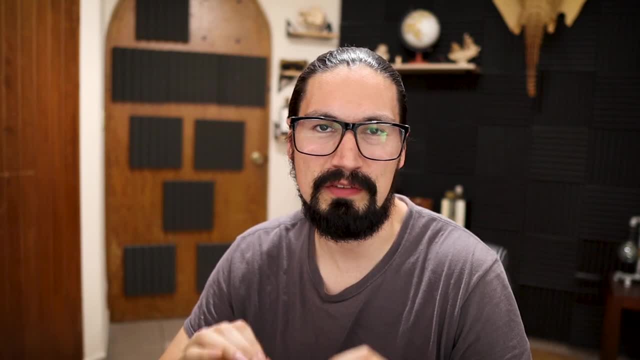 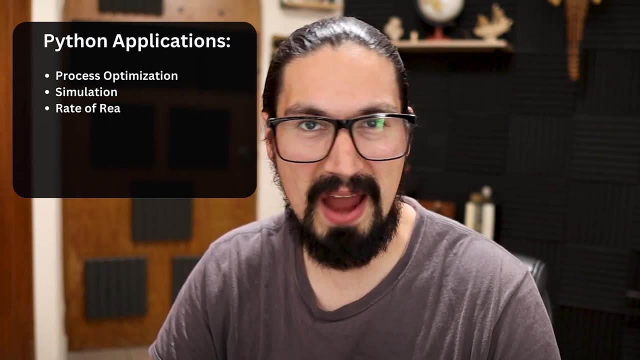 if you want to learn a programming language, Python will be a good fit for you. Whether you are interested in process optimization, maybe process simulation, or maybe you want to improve the rate of reactions of your reactor with simulation, or so maybe you want to improve. 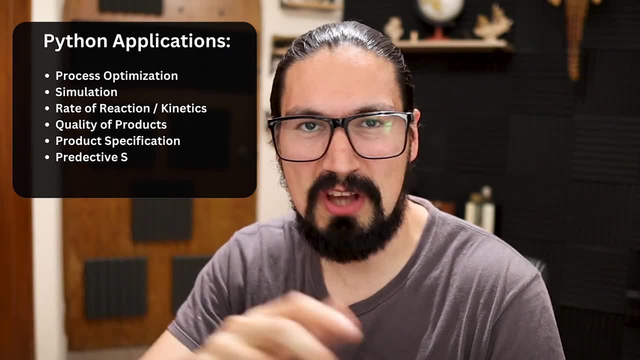 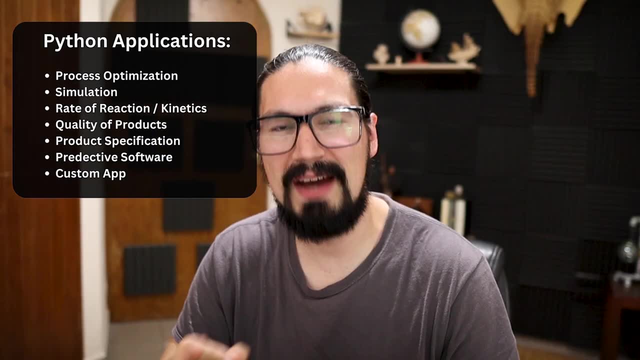 the quality of your products. maybe you want to create a predictive software for certain type of processes, even certain type of input, or maybe you just want to have a custom software for yourself, right fit for you. Now, as with any video guys, please let us know in the comment section. 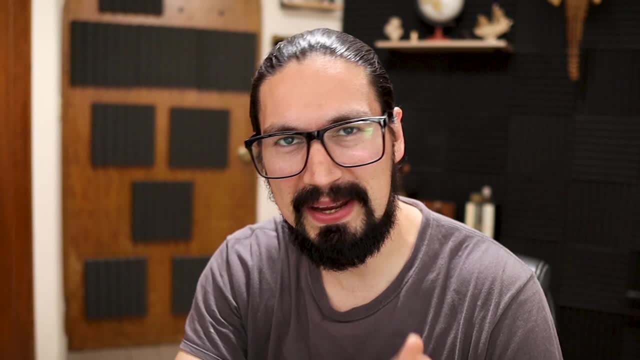 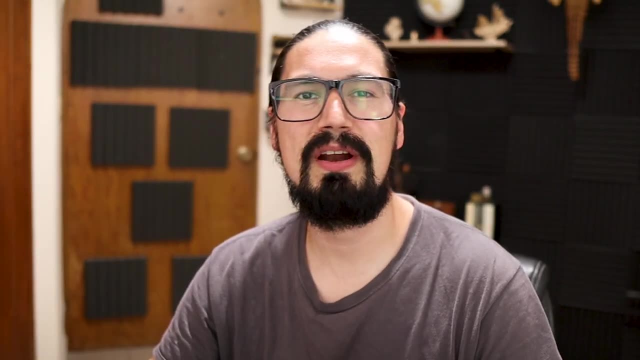 if you have already worked with Python, specifically in the chemical industry, What have you been doing? Have you used it to do a lot of data analysis? Maybe you use it for machine learning, Maybe you already use it for control loops or automation processes, or maybe you just 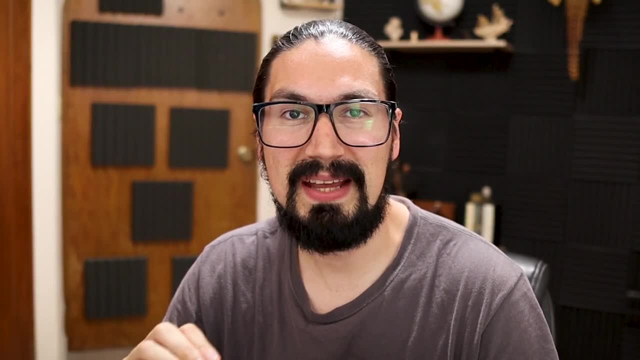 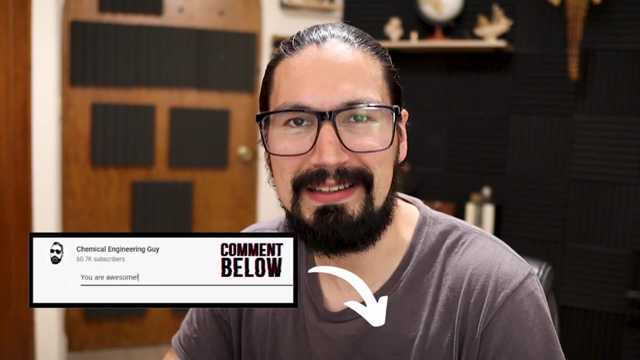 use it to have a software of your own. Whatever the case it may be, we are going to appreciate if you let us know what are the actual applications of Python in the chemical industry. On my behalf, that will be it, guys. I'll see you in the next video. 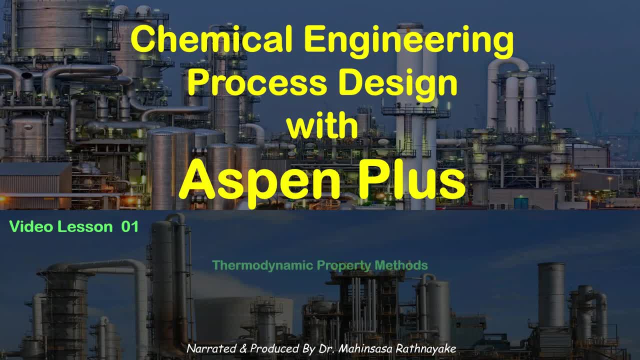 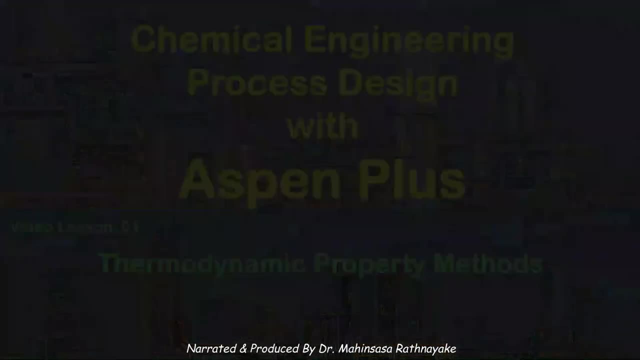 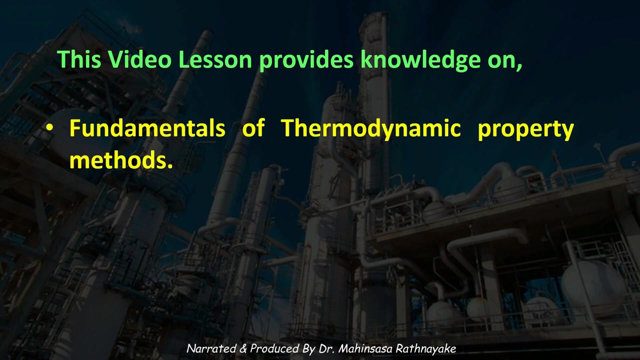 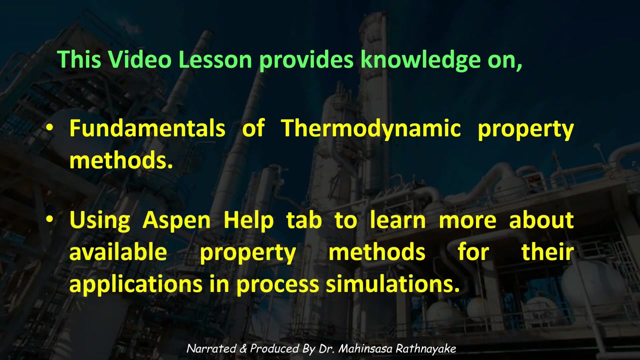 Hi everyone. Welcome to the chemical engineering process design learning videos with Aspen Plus software. This is our first video lesson. This video lesson provides you knowledge and skills for fundamentals of thermodynamic property methods and, using Aspen HelpTab, to learn more about available property methods for their applications in process simulations. 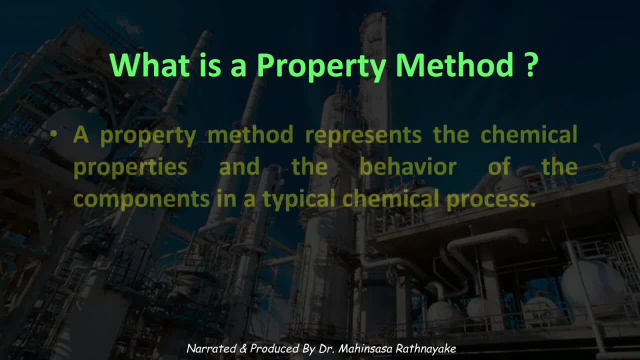 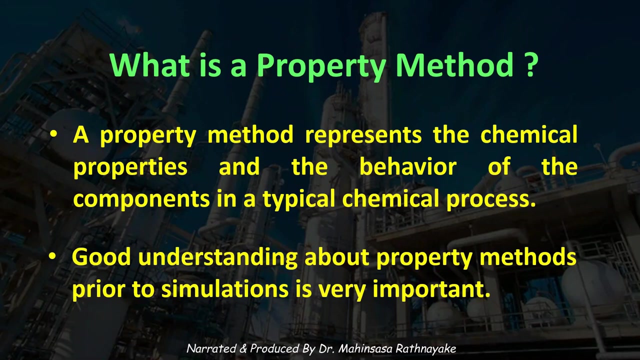 First let's get familiar into fundamental theory of thermodynamics. A property method represents the chemical properties and the behavior of the components in a typical chemical process. In other words, property method decides the accuracy of your chemical process simulation. Therefore, you must obtain a good understanding about property methods prior to simulations. 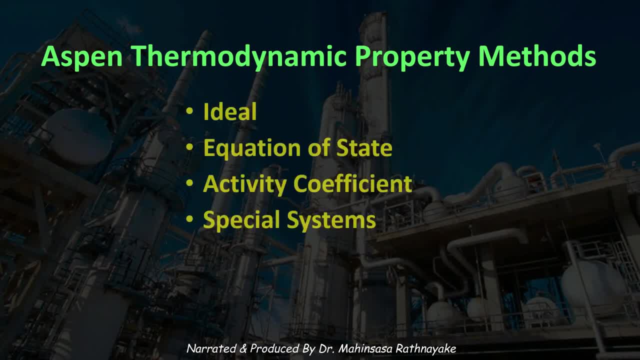 Aspen Thermodynamics is a technology that is used for the development of chemical properties. The thermodynamic property methods can be classified into four major groups. They are ideal property methods, equations of state activity, coefficient methods and property methods for special systems. When you become more capable of the Aspen software, you can even modify or create property methods in simulations for your own process applications. 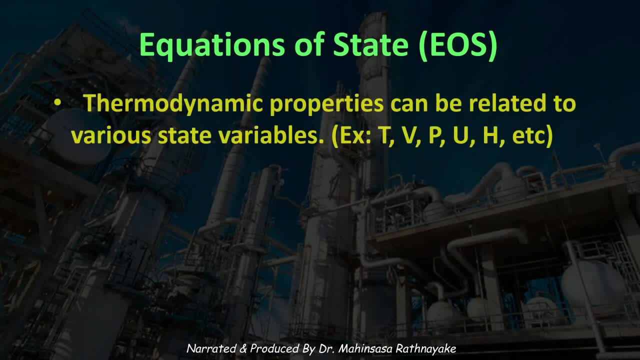 What is an equation of state? A cool death used for trial simulation can be called an ideal gas flow or ideal gas vacuum. Air pollution, air multinational emission, atmospheric, ambient. second flow. HR Known was identified as 210%. Temperature volume, countries, ah, internal energy and so on.